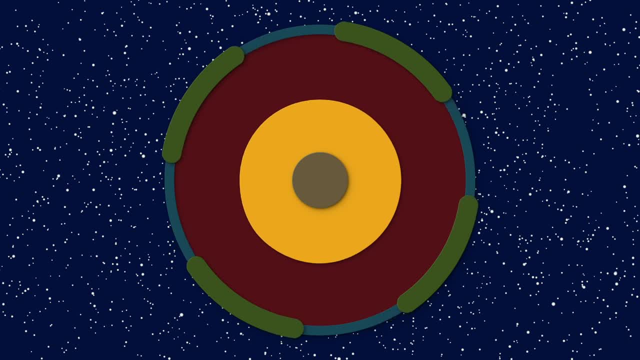 core, which is made up of liquid iron. When the earth spins, the outer core kind of sloshes around. This is what's responsible for generating the majority of the earth's magnetic field, which protects us from all kinds of energy. This is what's responsible for generating the majority of 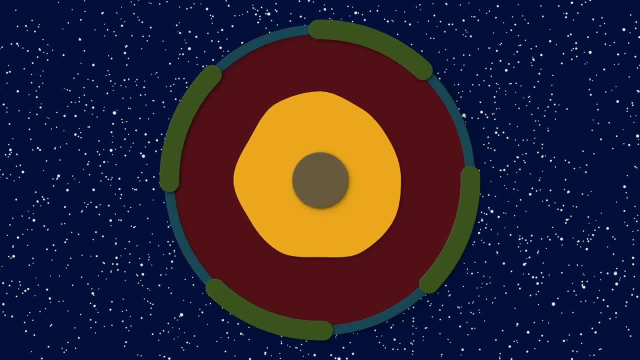 the earth's magnetic field, which protects us from all kinds of energy. This is what's responsible for generating the majority of the earth's magnetic field, which protects us from all kinds of extraterrestrial radiation. Without it, life on earth would be impossible. Thanks, outer core. 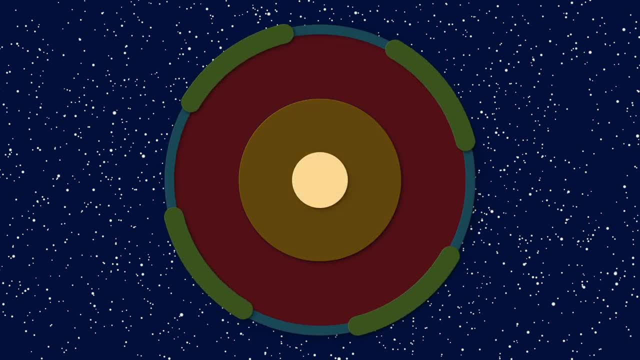 Finally, the earth is hard core, That is, it has a hard or solid inner core, again made up of mostly metallic elements like iron and nickel. It's super hot: over 5,000 degrees celsius- That's about the temperature of the sun, Even though it's the 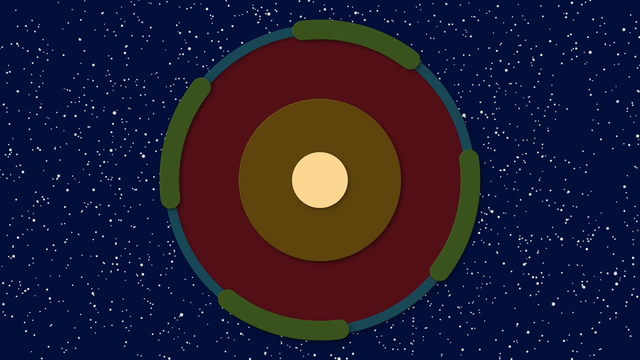 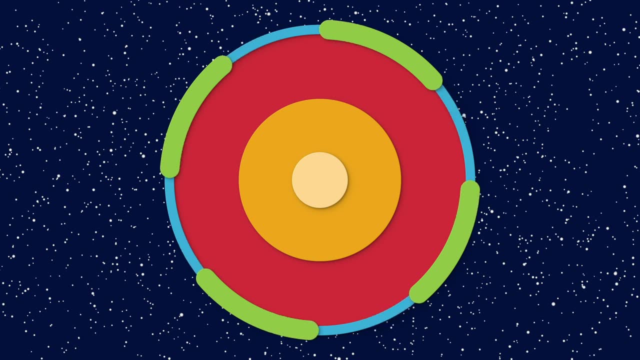 smallest layer, only about one percent by volume. the inner core plays a key role in helping the outer core generate our sweet, sweet magnetic field. If you're wondering what the structure of the earth looks like, that's it. And just so you know, the structure of the earth diagram. 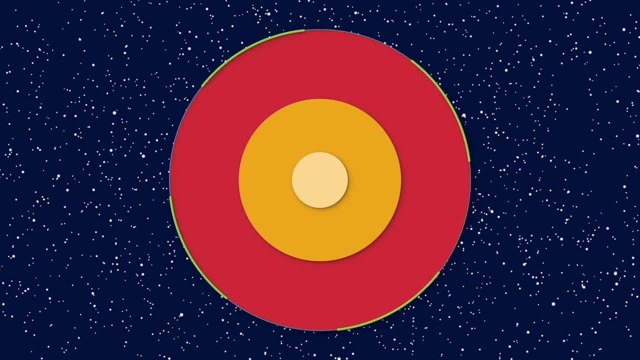 really looks kind of like this. The structure of the earth diagram really looks kind of like this. We just exaggerate the layers to make it easier to see. That's all great, but how do we know the structure of the earth? Have humans actually traveled to the center of the earth? The answer: